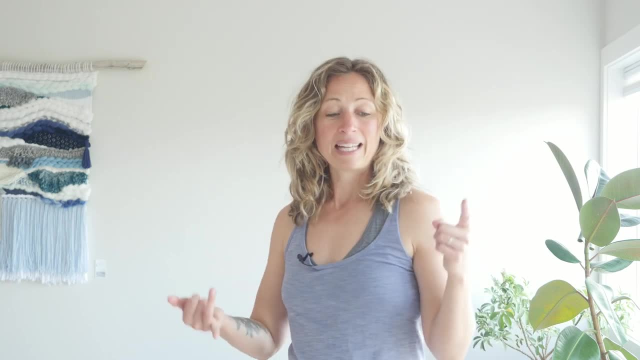 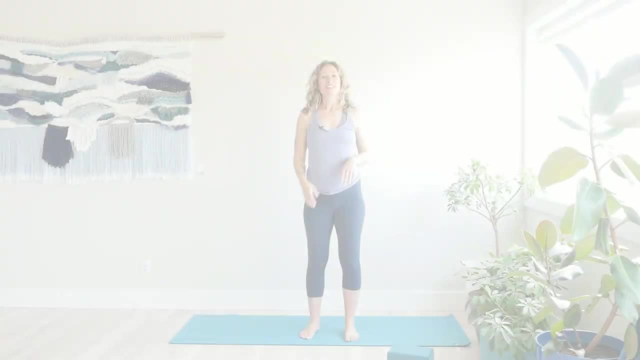 but move and learn with me. So you're going to need a yoga block and a wall if you need extra support. But let's go explore some tree pose variations. The good news is, with balancing poses, they're probably one of the best ones that even if you're using the same cues each time, 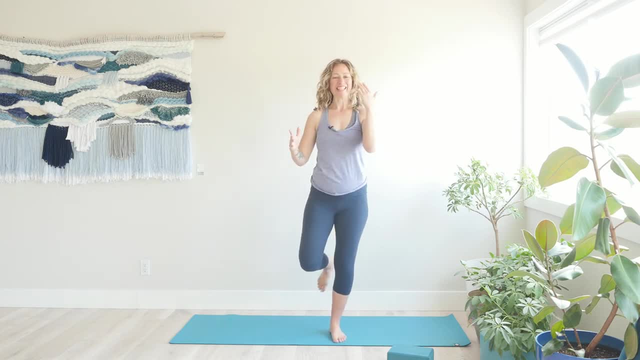 the very nature of balancing is that you're going to be able to do a lot of different things. I have a little bit of experience with balancing poses. I love it, So one thing that's really great about balancing poses is you're going to be able to get your brain 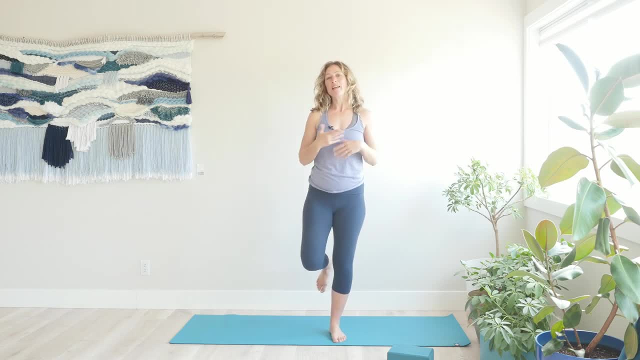 and body really kicked on and focused, But we can uplevel that, of course, by exploring more active movements in our balancing pose, And so active movements means that- and in this case, active movement means that we're going to actually work on what this leg is doing. 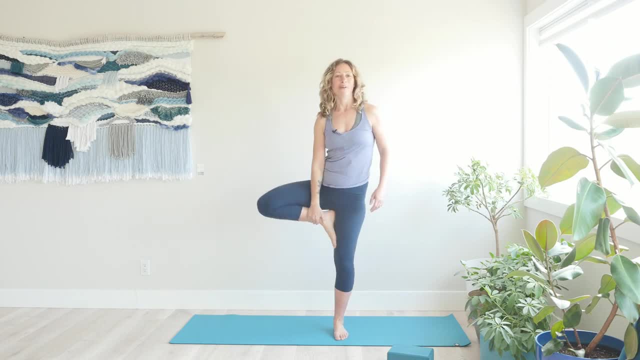 the leg that normally goes here or here or here, wherever it is for each of us, And we usually just keep a balance. It's a nice little movement, It's a cat's paw movement And that's how you're going to get all the energy up and running from managing That's okay. You just bring your balance to an even. 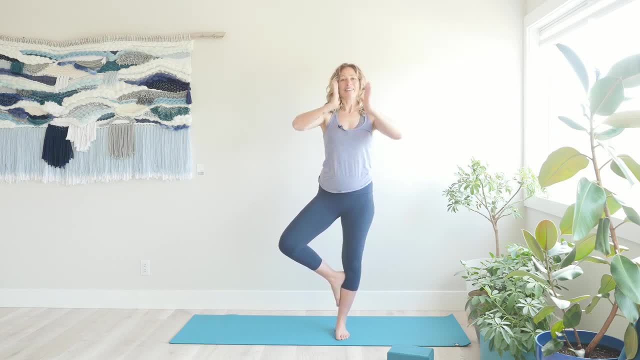 that foot pressing against the leg and holding and the arms come up. however, we do it, But what we're going to do is activate that and kick that on a little bit more. So what I like to do is use the standing. So you're going to stand on one leg, you'll bring one knee up and then turning. 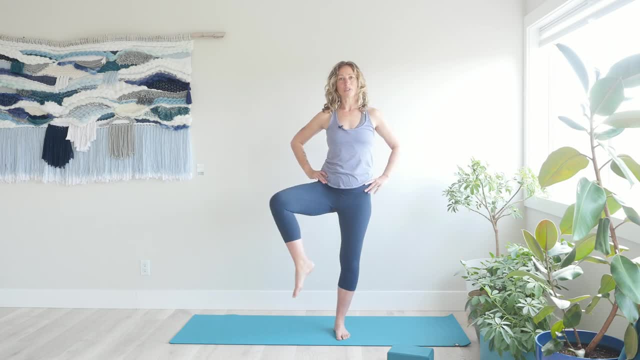 having your hands onto your hips. This is a beautiful opportunity to learn about hip mobility. while standing on one leg, See how that's good for your brain. So hip mobility means that you're going to keep your pelvis still and try to move your leg in and out. Now, if this is really 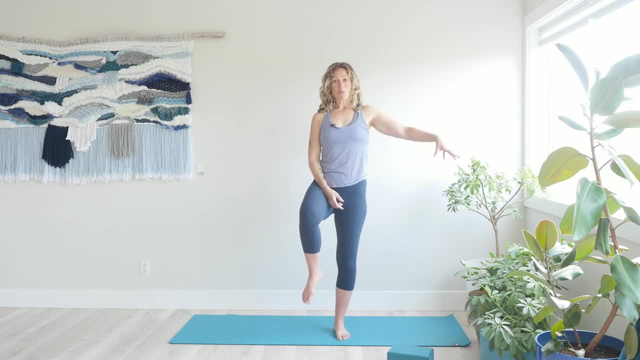 challenging for your balance. grab onto a wall, grab onto a chair and you can still absolutely get the benefits of this. And the next thing that you want to do to up level this is to not place your foot on your leg, So you're going to still try to move the knee out to the side. You're 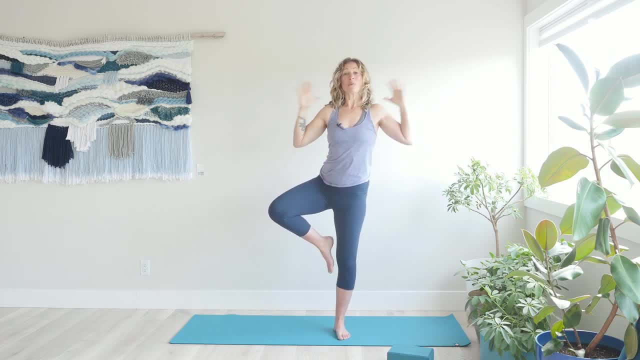 going to put your foot on the leg, but now you're not putting the foot on the leg, And holy guacamole, I don't know about you, but wow, is that ever a beautiful way to strengthen? So if you're a yoga, 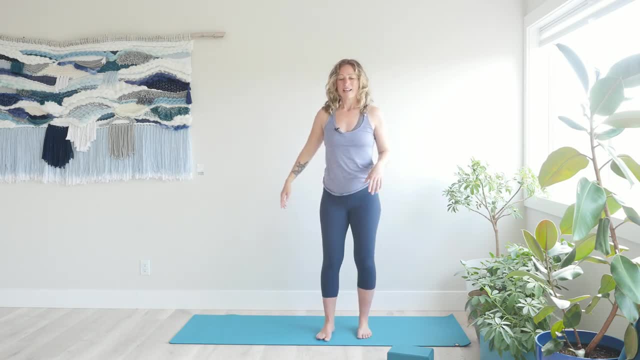 teacher, especially watching this, looking for new ideas for your classes. and if you're fine that people are getting kind of bored, well, this is going to unboard them, make them not as bored Because, all of a sudden, if we have to do it in a different way than what we're used to, 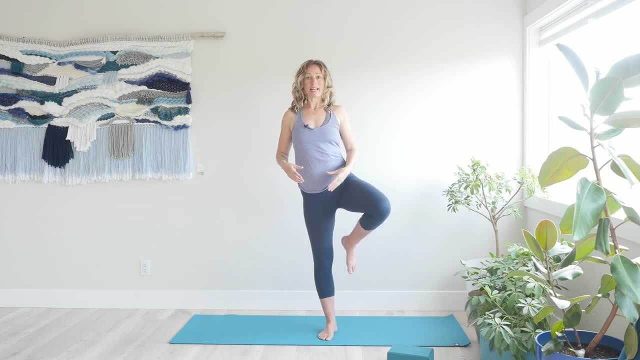 the brain immediately goes: oh, here I am. I have to work a little differently, So that's one thing that you can do. You can do a lot of fun stuff playing around with the leg. You can do hip circles like that and then eventually have. 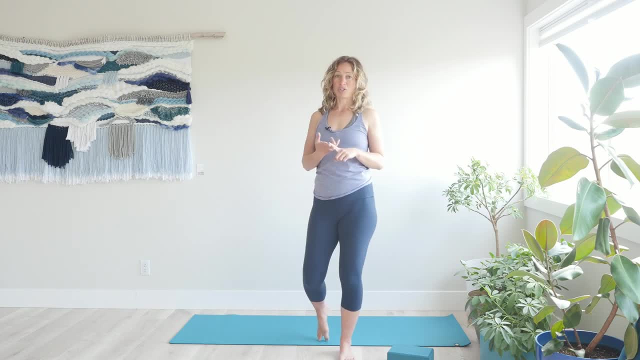 them here. Even another little option too, to pare that back a little bit is if people always have the same spot that they put the foot on the leg. So a lot of us will grab the ankle, we'll bring the foot as high up the leg as we can go, and then there's that pose. Now, if you've done, 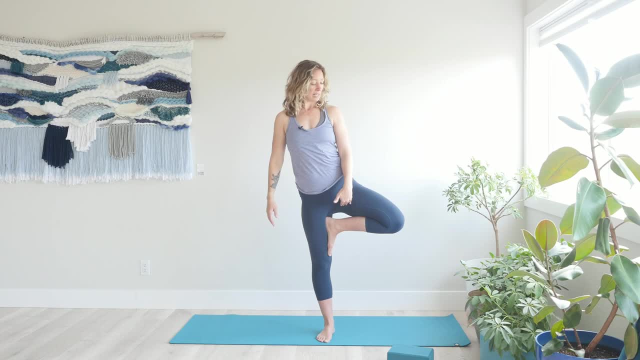 this pose this way the same time. every time you do it, the muscles are used to this position, So there's benefit to having the leg even just slightly lower. So if you're not ready to completely change everything, at least change the angle or position of where your leg normally is. 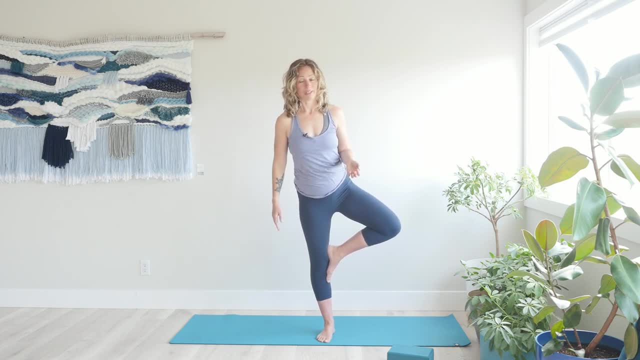 Because, guess what? You are not a better yoga person if you can get your leg here. You're not a lesser yoga person if your foot is down here. The end goal is not to have some sort of picture perfect pose at all, my friends. The end goal is: 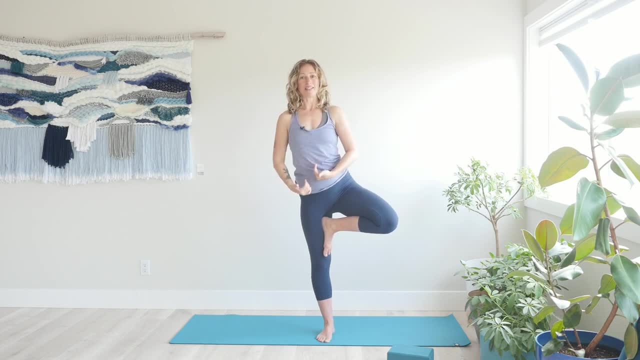 to keep ourselves awake and aware and engaged fully and present in our body, in our breath, in our mind at any given time. So when we have an opportunity to move in a different way than what we're used to, we're immediately engaged, We're immediately reconnected in a completely 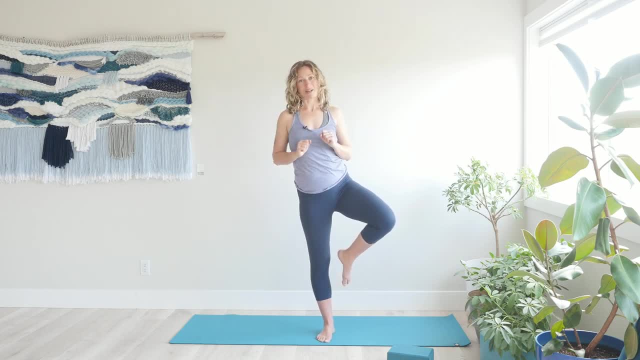 different way because it's unfamiliar, And that's where the benefits are. So let's do one more fun tree pose exploration here to keep that sense of variety and diversity, different ways of movement, into our mind and body, And I'm going to this. one requires having a block, And I'm going to recommend that it's a foam block. 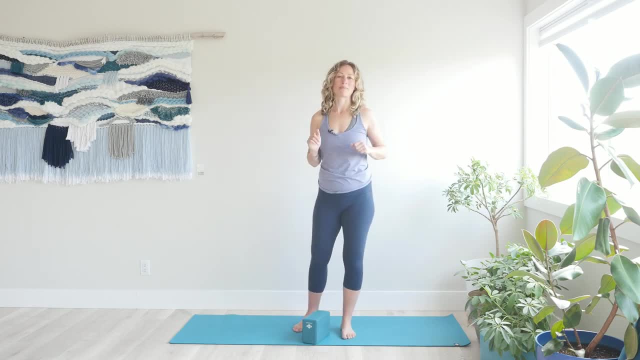 If you use one of the wooden or cork blocks, you'll see in a moment why that might be a little more challenging- not impossible, but just more challenging- And what we're going to do here is bring the foot to the block and the block by your leg, And then this is a really fun one, where you